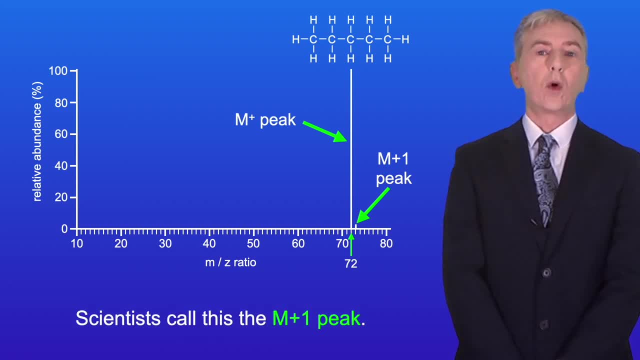 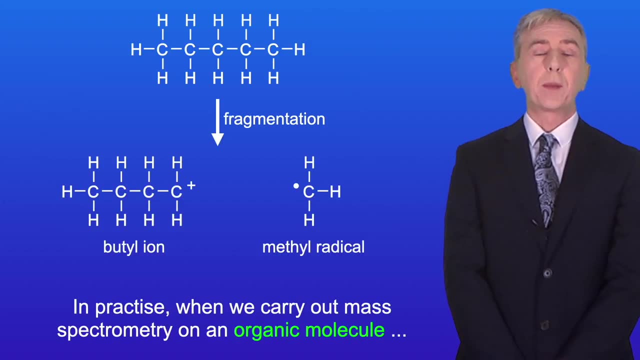 of carbon atoms. Scientists call this the M plus one peak, and this does not play a role in our analysis of the spectrum. Now, in practice, when we carry out mass spectrometry on an organic molecule, we get a range of different peaks. That's because organic molecules break up or fragment in the mass spectrometer. 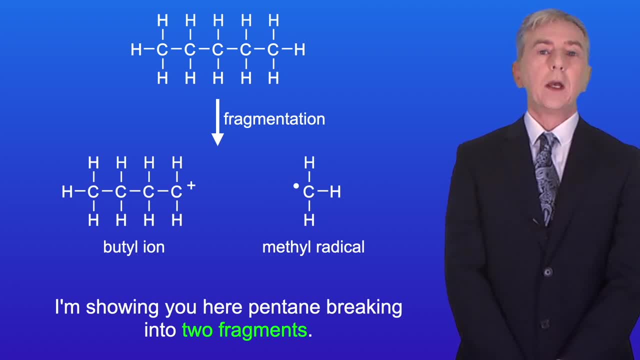 I'm showing you here pentane breaking into two fragments. When fragmentation happens, a bond breaks and we form an ion and a radical. Only the ion can be detected by the mass spectrometer, in this case the butyl ion. However, bear 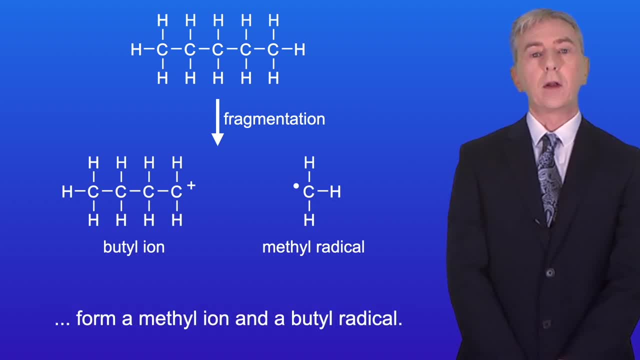 in mind that the fragments could just as easily form a methyl ion and a butyl radical, So in practice, both fragments will be seen on the mass spectrum. I'm showing you here the fragments produced by breaking carbon-to-carbon bonds in pentane. 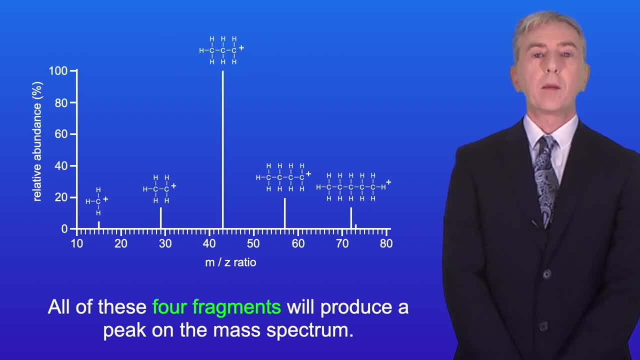 All of these four fragments can be seen on the mass spectrometer, but they can't be seen on the mass spectrometer. I'm showing you here the fragments produced by breaking carbon-to-carbon bonds in pentane. All of these four fragments will produce a peak on the mass spectrum. 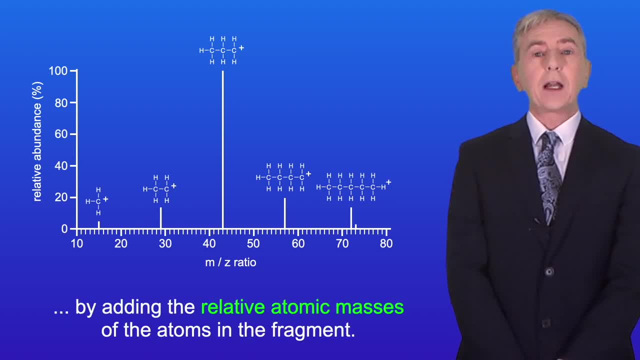 We can work out the MZ-ratio of each peak by adding the relative atomic masses of the atoms in the fragment. Now there are a couple of points to notice about this. Firstly, some fragments are more stable than others, so each fragment will not have the same abundance, And secondly, 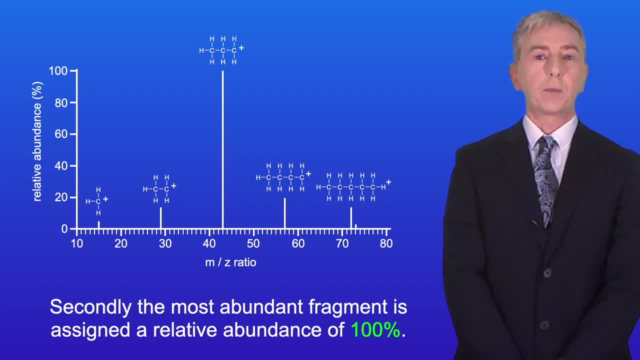 the most abundant fragment is assigned a relative abundance of 100 per cent. Scientists call this the base peak. here the most abundant fragment is the propyl ion. Now, in practice, the carbon to hydrogen bonds can also break in the mass spectrometer, so 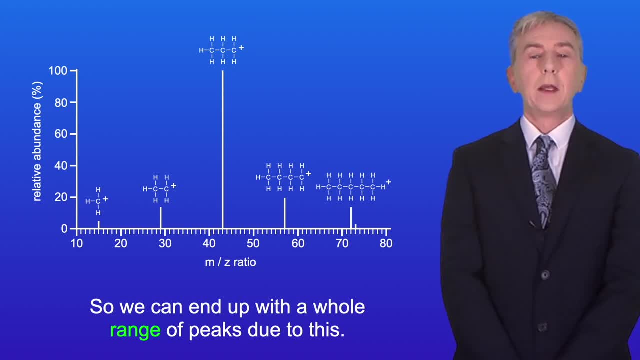 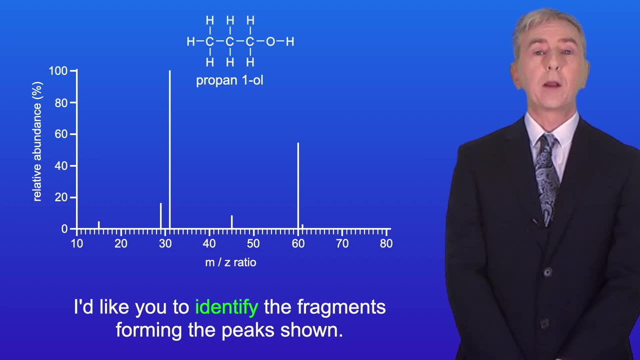 we can end up with a whole range of peaks. due to this, I'm showing you here the simplified mass spectrum for propan-1-ol. I'd like you to identify the fragments forming the peaks shown. so pause the video now and try this yourself. 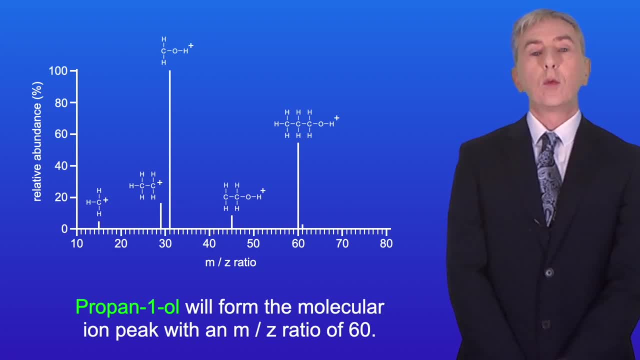 OK, so propan-1-ol will form the molecular ion peak with an MZ ratio of 60.. The other peaks are caused by the fragments shown. Again, I should point out that I've not included any fragments formed by the breakage of a.